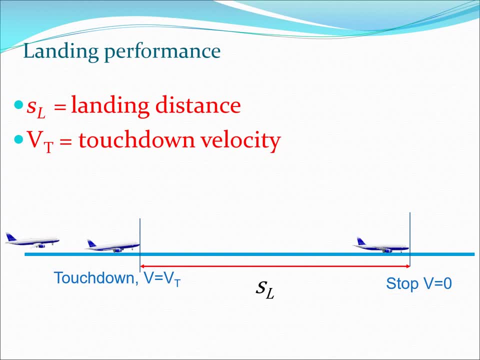 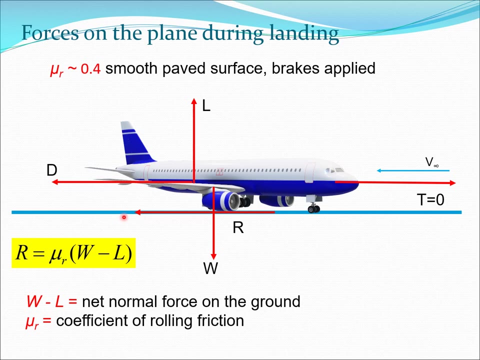 the runway length you need at a particular airport, because if you do know the different type of aircraft, you know that you are going to land at that airport. then you can come up with that runway length. So let us look at the aircraft and look at the different forces which act on it. So I've 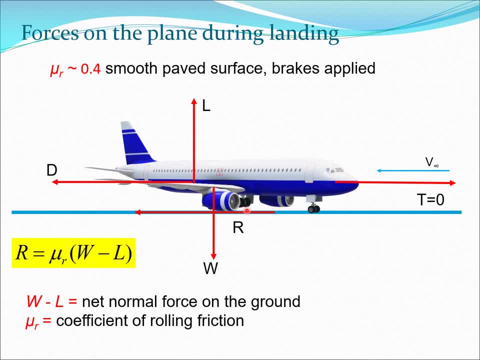 drawn this aircraft here, a schematic, and you can see here that because there is a velocity coming from the front, you have the lift, you have the drag, you have the weight acting downward and also you have the lift, The force. here are the reaction. Now the reaction is going to oppose the direction. 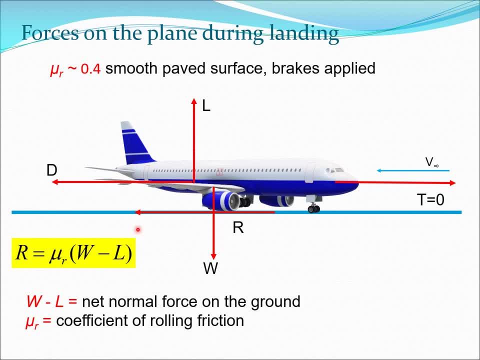 of the aircraft motion and this is coming because of the presence of rolling friction. So because the aircraft has wheels, you are going to encounter this rolling friction and this is equal to mu r into w minus l. So here, w minus l is the net normal force on. 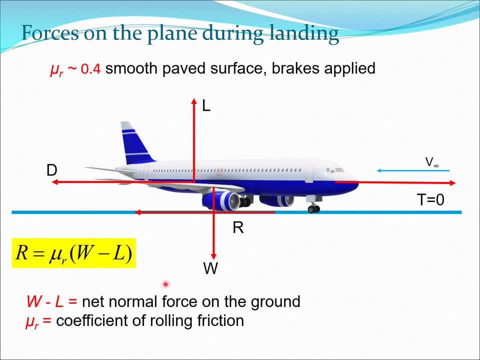 the ground. So it's the weight minus the lift, and mu? r is the coefficient for rolling friction, Which is, in the case of an aircraft, if you apply the brakes, it's going to be something like .4 for smooth paved surface. Now, do remember that when the pilot is trying to 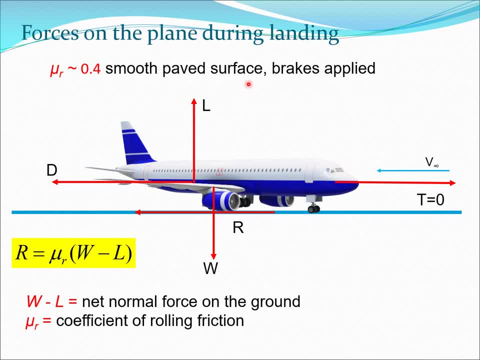 land the aircraft. he has applied the brakes, So the rolling friction is much more than in the case of takeoffs. So in the takeoff case it was .02 and here it has gone up to .4.. One more thing to remember is the pilot is landing the aircraft, So he really does. 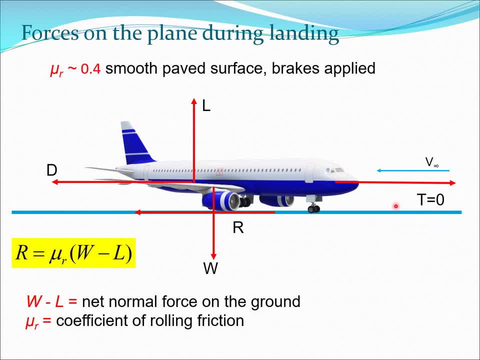 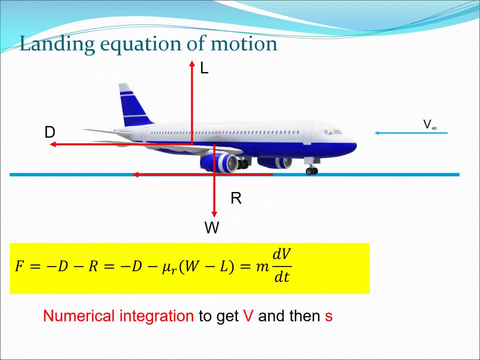 not need .2.. But in the case of the takeoff, he is not going to need .2.. He has a lot of thrust, so they often set the thrust vector to zero. so there is no trust acting on the aircraft. now, based on these forces, we can write the governing equation of motion for landing. 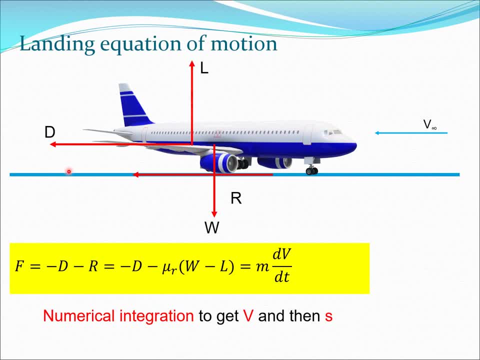 so the equation of motion is: force is minus t minus r. this is d minus mu t, w minus l, and this whole thing is equal to m tv by dt. so this is newton's law of motion, that mass into acceleration equals the force. now, if you had the variation of drag and lift with respect to time, 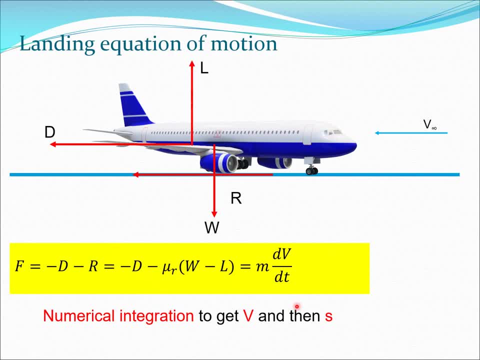 you could essentially integrate this equation, and numerical integration would tell you what's the velocity profile with respect to time and, if you obtain that, you could also obtain the velocity profile with respect to time and s, because the distance and velocity are related. now, this is the exact way of doing this problem, but what we are going to do is we are going to 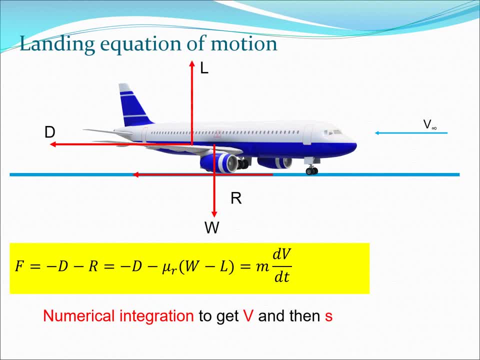 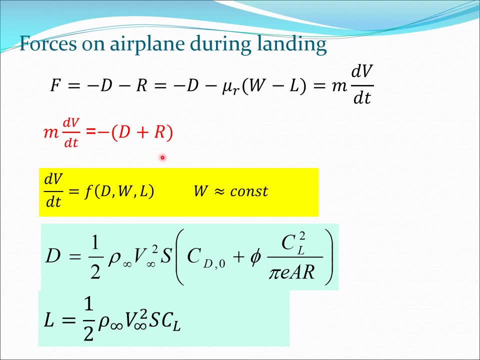 make a number of approximations and we are going to come up with a simple, closed form solution. so let's rewrite the equation here. so this was the equation of motion we had. m dv by dt is minus d plus r. now here we can clearly see that. 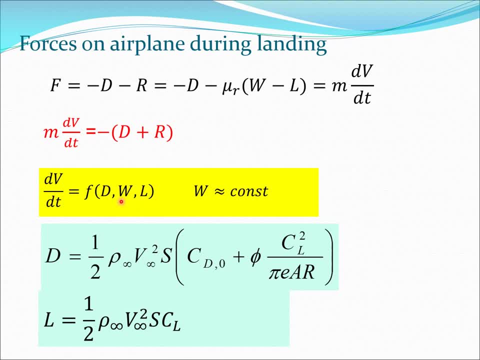 we have the velocity profile will be小 way. so if it 하는데 into the centre of the plane weight, this is more or less constant and therefore in this particular pattern i can put: i is the locked expression and therefore i can put in constant t. so here, subject to: 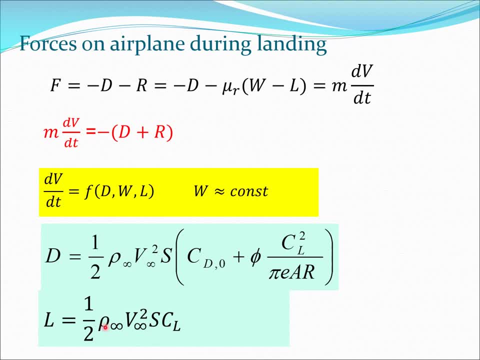 the associated vector is the load, and so, but, but as i just explain that, the weight became more or less constant for everything but some of the things we have, we have same graph, but definitely where rho is the density of air, v is the velocity of the aircraft, s is the area of 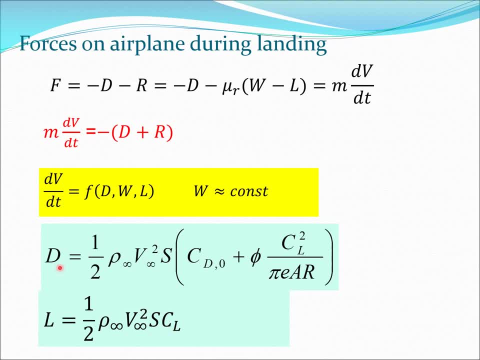 the wing and c? l is the lift coefficient. If we look at drag, we now see here we have c d or the drag coefficient, which has two parts: the c d 0 part is the 0 lift drag and the c? l square by pi e. a r is the induced drag part. So do remember a? r is the aspect. 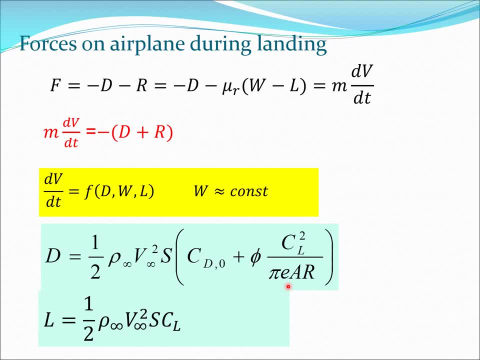 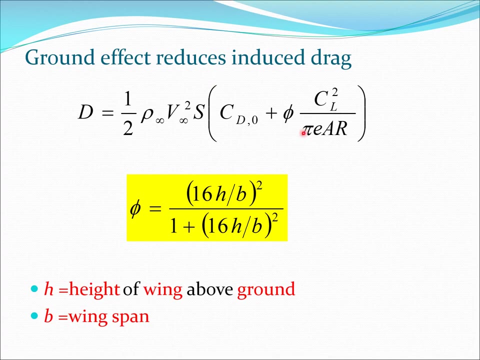 ratio of the wing. v is the Oswald span efficiency factor, and phi is a factor which comes in because we are near the ground and so ground effect is going to become important. So what happens is that ground effect typically reduces the induced drag. So this factor- 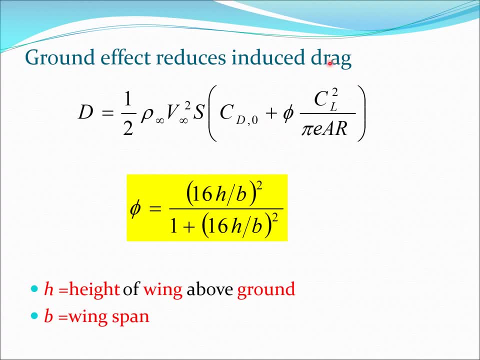 phi. here this is less than 1 and we multiplied by the induced drag factor c, l, square by pi, e, a, r, and so this is going to reduce the induced drag. So the factor phi is given by this equation here, which has been obtained from fluid dynamics. 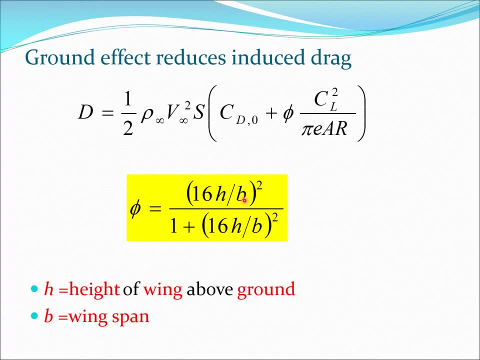 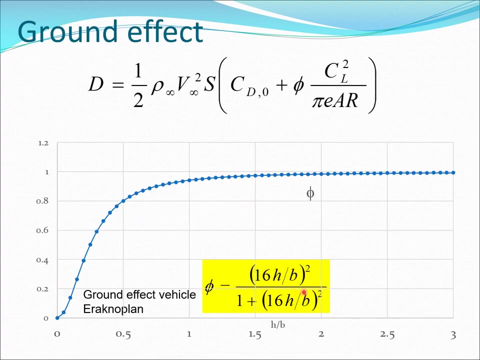 theory and this equation says that phi is 16 h by b square divided by 1, plus 16 h by b square, where h is the height of the wing above ground and b is the wing span. So if we were to plot this factor phi, which I have done here, So on the x axis I have h by b. 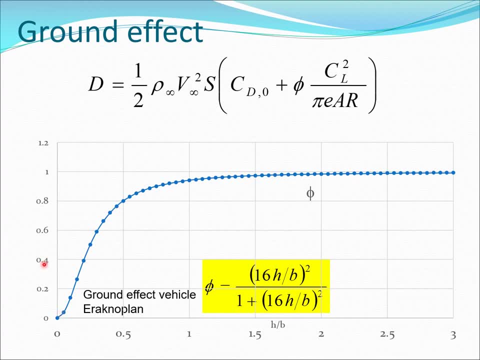 and on the y axis I have phi. you can see that there are many parts of the regime where phi value is quite less. So essentially, if h by b is something like 0.5 or below, then the value of phi is quite less. it can be as low as 0.2 and so on. Now, beside the importance, 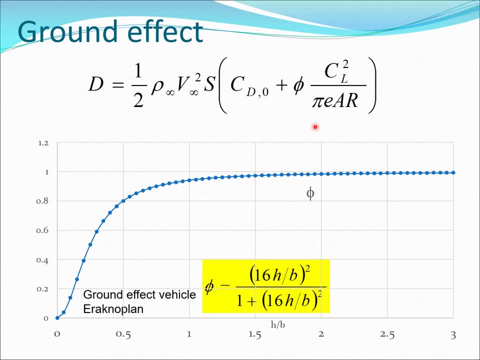 of this during the runway takeoff and landing. this kind of phenomena is also used by many vehicle, such as the ground effect vehicles, and these are essentially airplane like systems which fly very close to the ground. Very often, these are vehicles which fly on the sea or 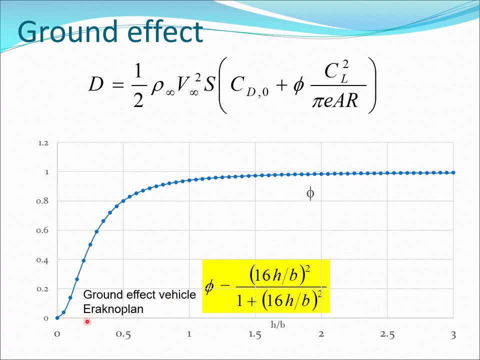 just on top of the sea. So sometimes they are all known as the irachnoplans. so these kinds of vehicles were often developed to fly in regions where there is a large sea. may be, there are a lot of islands in between. Cavaleness素 as the in most cases So theseido modules during aорот- докумώ. 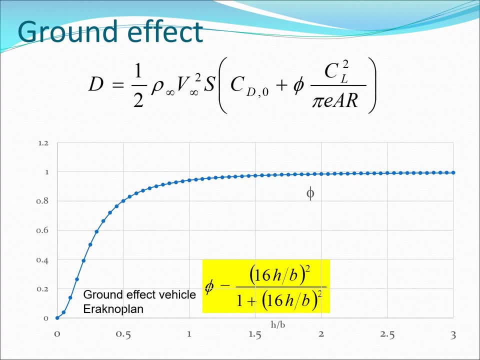 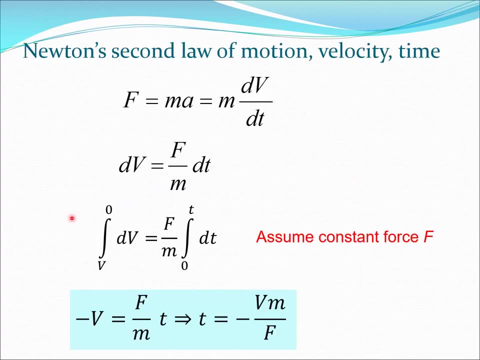 diacno plans can travel between them at a much reduced cost because what's going to happen? the induced drag is going to be much less So. now let's get back to the Newton's law of motion and we are going to derive some expressions for the time taken, the velocity and the distance. 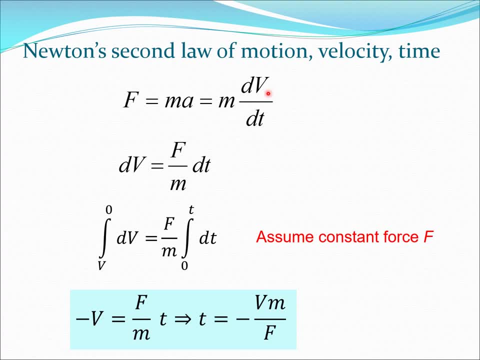 So we start with f is ma, is m into dv by dt. So we can write dv as f by m into dt, and then we integrate these two sides from v to zero and zero to t. So what this says is that at the velocity v, that means when you are landing the aircraft, your time is zero. and at the end, when 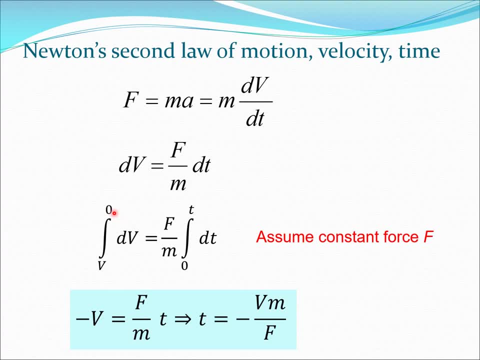 you have come to a stop on the runway, the velocity is zero and the time is t, and this can be done if we assume constant force f. So that allows me to bring this f out of the integral sign, and I am also assuming that mass is constant. So in this kind of situation I can integrate this and I get two. 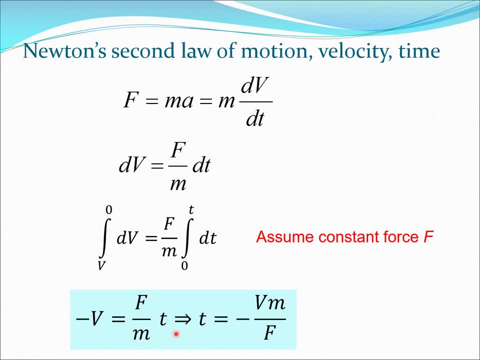 equations I get negative: v is f by m, t or t is minus v, m by f. Now this minus sign comes in, because in this case what happens is that the force applied is a negative force, So actually the time is going to come out positively here. Now, from the same equation, I am going to try to 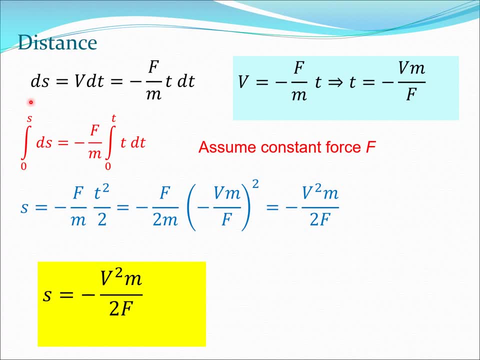 calculate distance. So again, the basic formula for distance is: ds by dt equals v, So we get: ds is v, dt, and this becomes minus f by m, t, dt, which then lets me calculate the distance s. So what I do is I integrate this from zero to s and from zero to t, So at time, t equal to zero, the distance is zero. 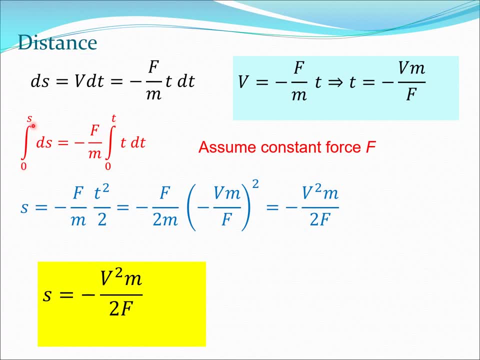 at time t equals t. the distance is s. I put the value from t from this equation here. So t is minus v m by f. So when I bring this equation here into s, I get this equation which is: s equals negative f by m, t square by two. 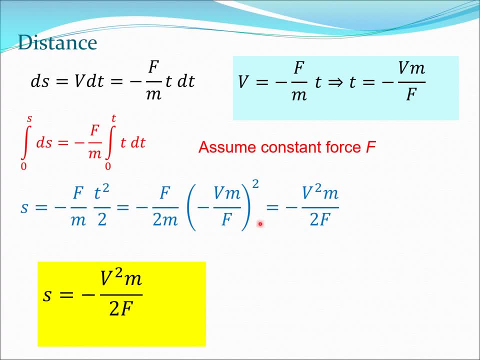 and then I substitute for t, I get this here, and so I finally get the equation that s is minus v square m by 2 f. So once again, remember that this equation assumes that I have constant force, f, and also the force is negative. in this case, therefore, s is going to turn out to be: 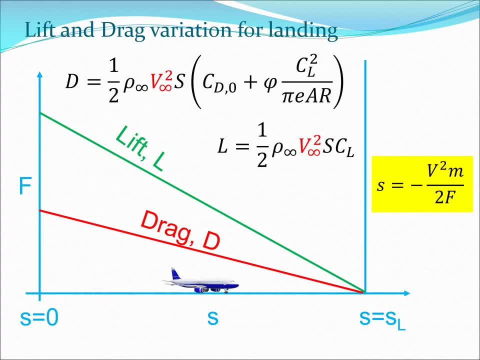 positive. Now, if you are going to plot the different forces to get a physical feel for them, so let's start with the lift and drag variation. So if I look at lift and drag, remember initially, at s is zero, the plane has landed with a pretty high velocity and so there is going to be 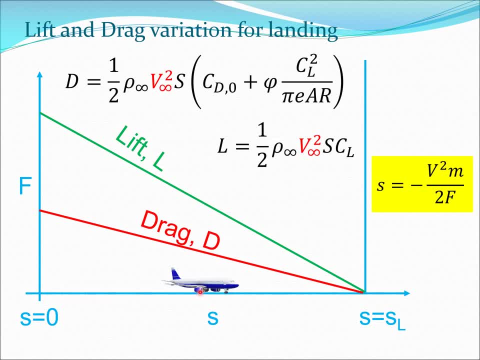 substantial lift and drag, and as the plane taxis down the runway and comes to a stop at, s is equal to sl. the lift and drag are both going to become zero, So they are essentially directly proportional to v square, and from this equation we can see that s is. 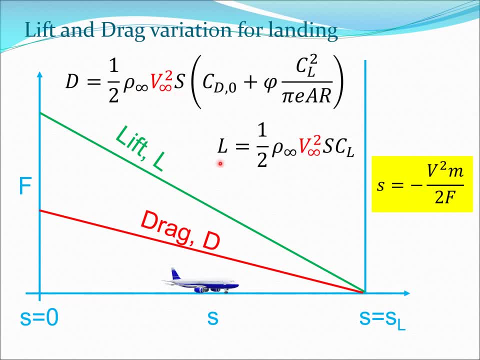 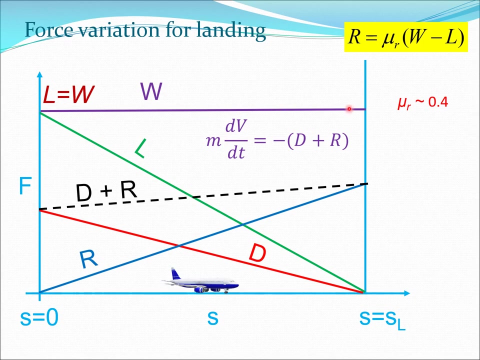 proportional to v square also. So essentially, d and l vary linearly with respect to s. So that's why we have these two straight lines here and, of course, because you have wing sections which are typically designed for lift by drag maximization systems. Lift is much higher than the drag. Now let's add the next part here, which is the weight, So the 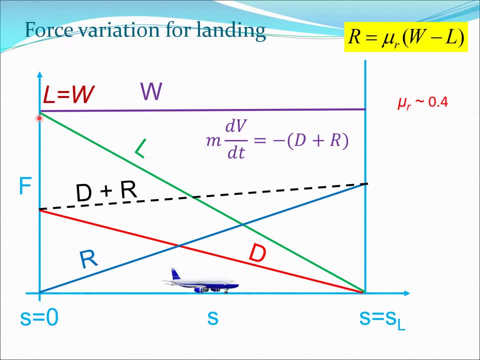 weight remains constant, and when you are landing the aircraft, we will assume that lift is equal to weight just before the point when you have landed and at the point this essentially holds, and so the lift decreases to zero, the drag decreases to zero, the weight remains constant, but the value of 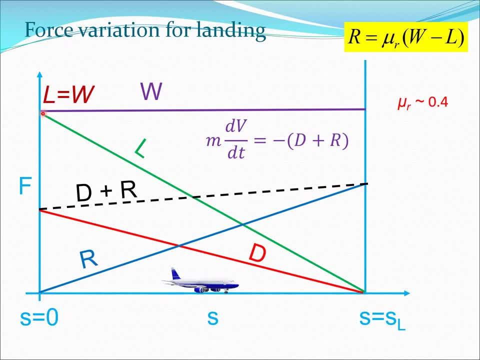 r goes up all the way here. Because what happens? that when you start this process at s equal to zero, lift is equal to weight, so r will be zero. that's the point here. and when you reach the point s is equal to sl. here, lift has. 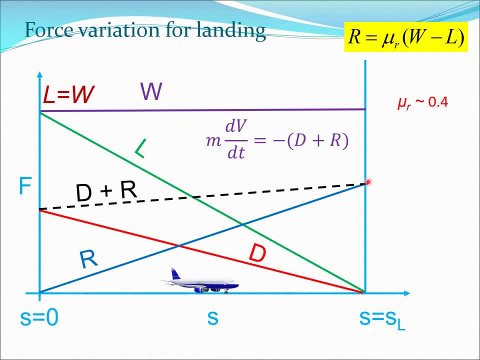 become zero. so you have simply mu r w. so you are at this point here. Also, remember that, since the pilot has applied the brakes and you are in rolling friction, mu r is 0.4. so actually this value is substantially larger than it would normally be if you did not apply the brakes, and so that's the point you get Now. next, 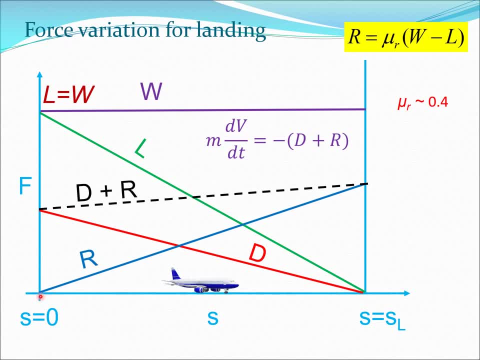 you can calculate d plus r. so here you can see that at s is 0 we have only d, r is 0. so you start from here, and at this point here you have only r, because d is 0. so d plus r essentially goes through. 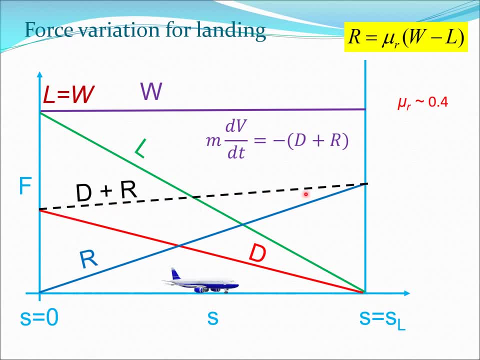 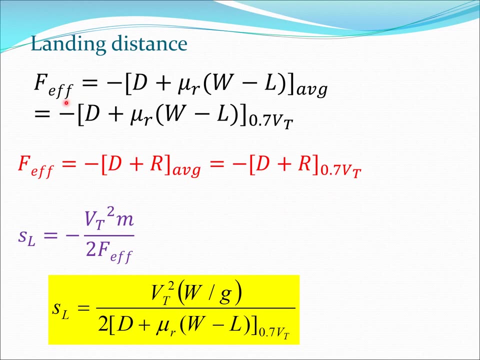 a variation like this. So this is the factor which we are concerned with: d plus r, because do remember that the equation was: m dv by dt equals minus d plus r. so now, in the previous equations, we talked about the force being constant. so what we are going to do is we are going to assume an effective 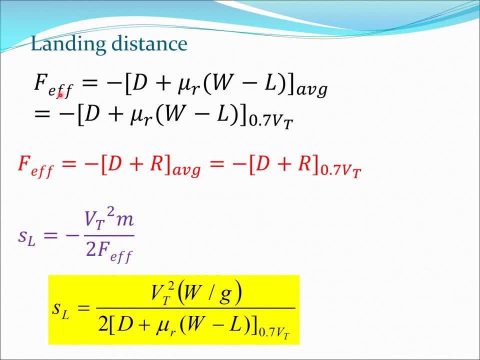 or average value of the force. So let's presume this effective force. this is minus d plus mu r w, minus l, the average value, and so I can write it in this form. and what we do here is that we take the value at 0.7 vt- remember, vt is the touchdown velocity- and then I can say that f effective is. 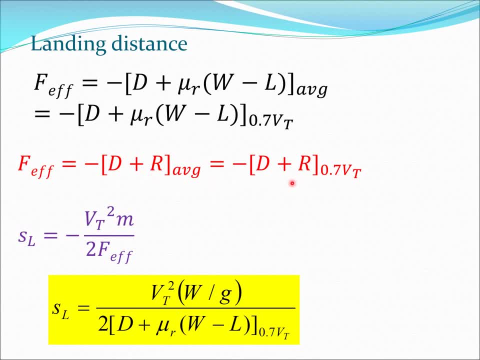 minus d plus r, the average value, or minus d plus r, 0.7 vt. Now I know the equation for s, so essentially I can get the value for sl. so to do that, I substitute: v is vt, that is the touchdown velocity, and I bring in the effective force, f. effective here. 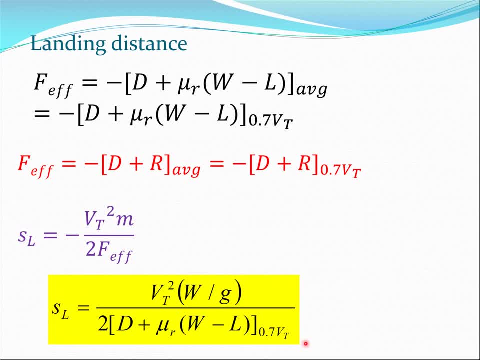 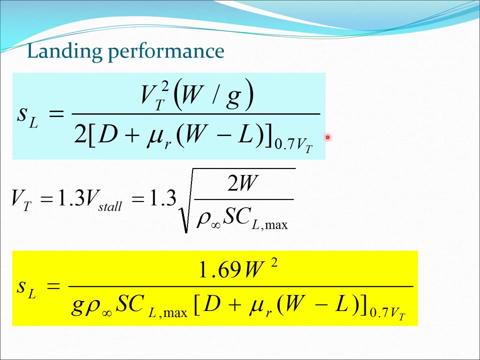 So I get this as the equation which I have put in this yellow box for s of l. so this is the landing distance. it's vt square w by g is the mass 2, and then this is the f effective value, which has been taken at 0.7 vt. So this equation is very important. so let's rewrite this equation. 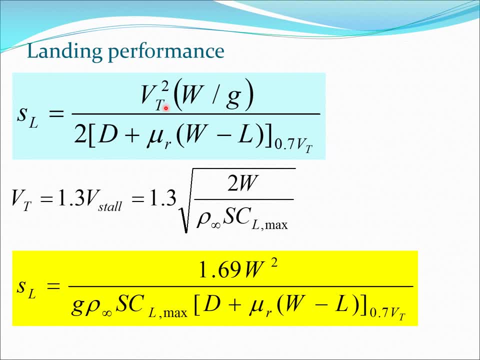 and what we do is we now get an estimate for vt. so what we are going to assume is that vt is 1.3 times v stall, so we can write it as 1.3 times root 2 w by rho infinity s, c, l max. so 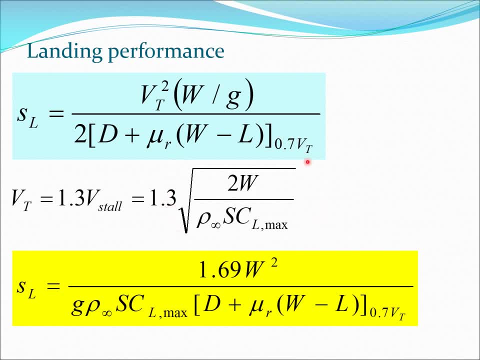 remember, the stall speed is given by this expression inside the square root here, or rather the expression in the square root here. So we clearly know that the stall speed is, of course, the lowest speed possible. so you don't want to actually reach it in flight, you keep. 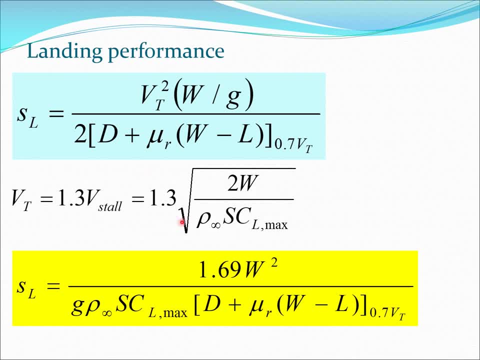 the aircraft at a speed which is slightly higher than the stall speed. so that gives you some margin of safety or factor of safety when you are landing. and then I put this value in sl, so I get this equation here. so vt square, so 1.3 get squared, so you get 1.69, you get w squared term, and then 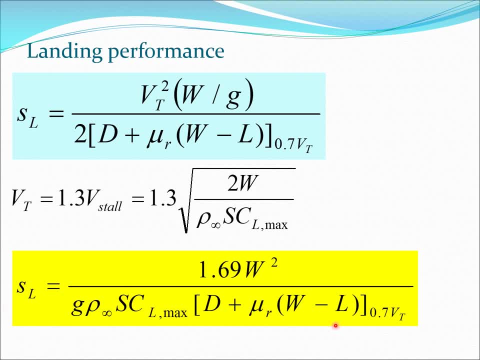 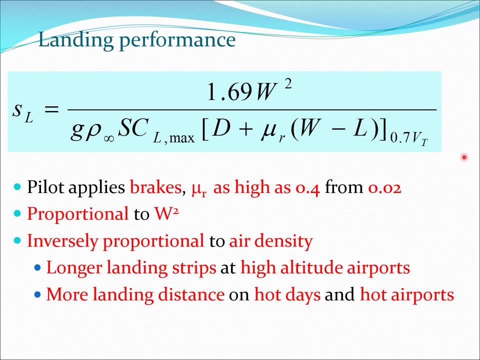 at the denominator. you get all these terms here. So this is the complete equation for the landing distance which we have obtained from the aircraft. So let's take a look at this math model and try to extract some physics from it. We can clearly see: 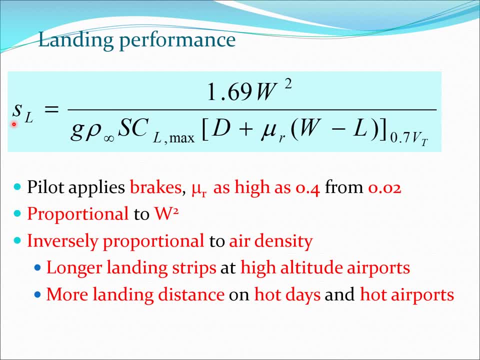 that the pilot would naturally want to reduce the landing distance as much as possible, so one thing he does is he applies the brakes, so the mu? r value would be high, for example 0.4, instead of it being something like 0.02 if the brakes are not. 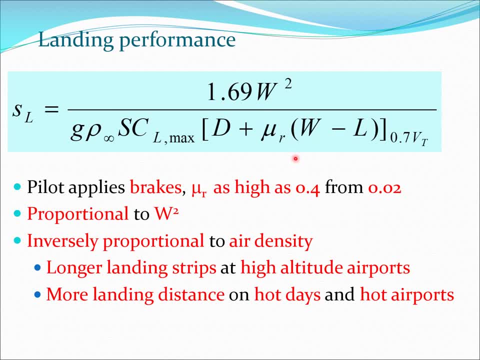 put in place, and so this is certainly going to improve the denominator term. Now we can see that sl is directly proportional to w squared, so if your aircraft has higher weight, for example, you are trying to land the a380, you may need a runway length which is much more than if you are lying. 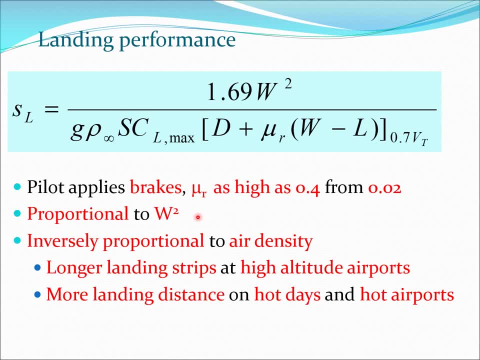 trying to land something which is much smaller, for example airbus a320.. Now we also see that it is inversely proportional to the aircraft weight. So this is going to be the length of the aircraft weight and the air density, because sl equals to 1 by rho. infinity here, or proportional to 1 by rho. 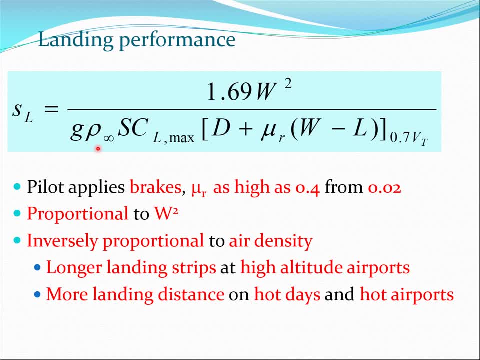 infinity. So what would happen is that the density of air is less, then sl will be more. So that happens in two situations. you can have airports which are situated high up, maybe in the mountains, and in those cases the landing distance is going to be more. Also, if you have situations where you 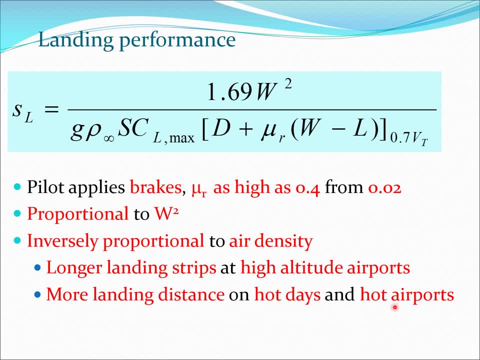 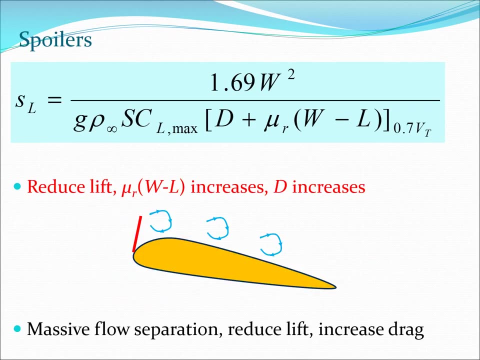 have hot days or cities where the airports are hot, For example during summers, then also you will require more landing distance. So these are certain things which need to be factored in, depending on the altitude and the heat your airport has to go through. Now there are some more ways to play around with sl or sl, and one of them is to use 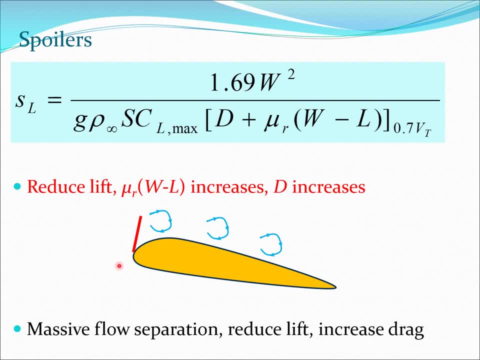 spoilers. So what spoilers do is that they reduce lift. So in front of the wing you put up something like this, It basically creates a lift. So in front of the wing you put up something like this and it does a lot of drag, causes flow separation. So what would happen is that d would increase and 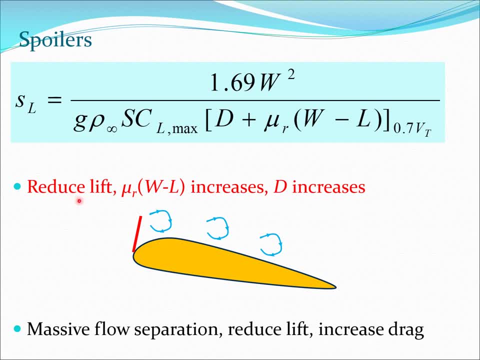 mu into w minus l would increase because lift would decrease. So that would mean this is increasing. this is increasing. So basically the denominator term is increasing, So the sl value is decreasing. So this is going to reduce the landing distance. So spoilers are important. 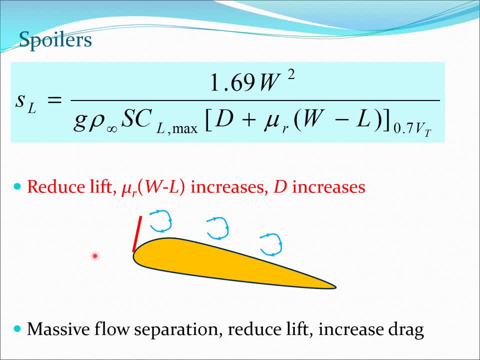 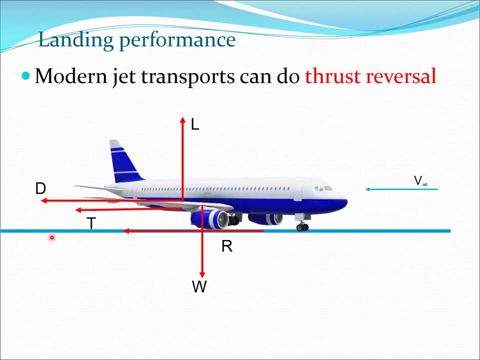 You will see that when aircraft are landing, the pilot is going to deploy the spoilers can often lead to lot of flow separation. You can often see these kind of complex vortex formations which are there if you are sitting near the window seat of the airplane. So one more thing which modern aircraft can do is they can do what is known as thrust reversal. 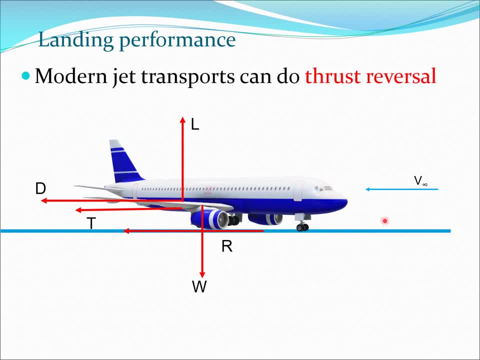 So in this case, what happens? the thrust, which is normally pointed in the forward direction, the pilot can send it in the backward direction, and this is certainly going to add to the resistance the aircraft faces. So the thrust, in this case, acts in the direction. 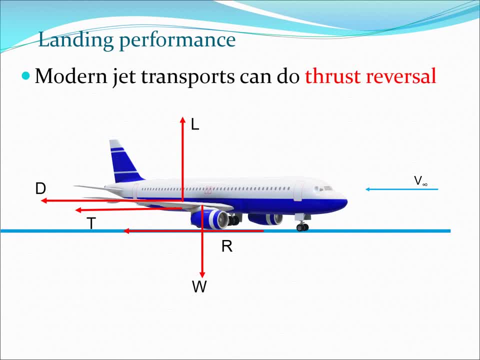 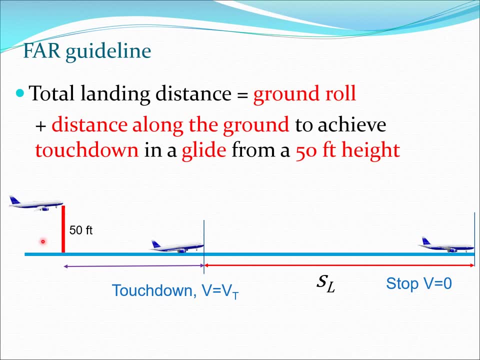 of the drag, and this can substantially reduce the runway distance, So this is something which can be used every now and then. Now let us come to the actual practical guidelines Now. today, what we did is we got an estimate for this distance s subscript l, which is the landing. 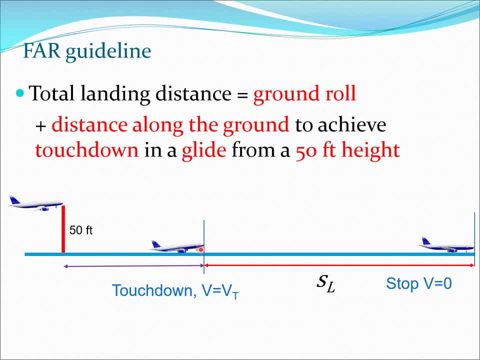 distance, So from the point where the aircraft touches the ground down to the point when it comes to a complete stop. But what is there is that, as far as the FAR guideline is concerned, the total landing distance is this ground roll distance, that is. 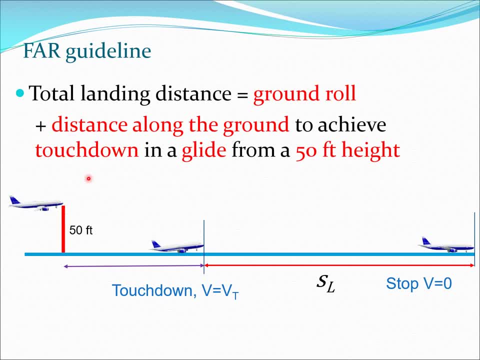 s of l plus the distance along the ground to achieve touchdown in a glide from a 50 feet height. So if you are at a 50 feet height here and maybe you need this much distance here to reach this point at touchdown, then this distance has to be added to the distance sl. So this is: 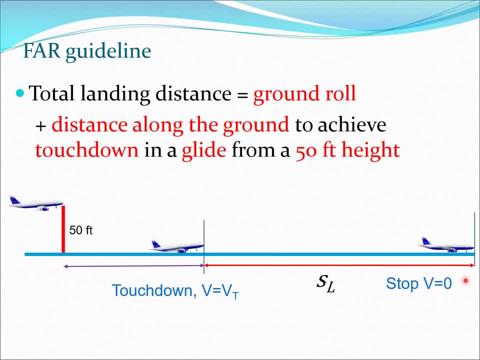 distance as far as the landing distance is concerned, and you have to make sure that the runway or the landing strip has this much distance so that you can safely land the aircraft- So this 50 feet is kept as a margin of safety or a factor of safety. 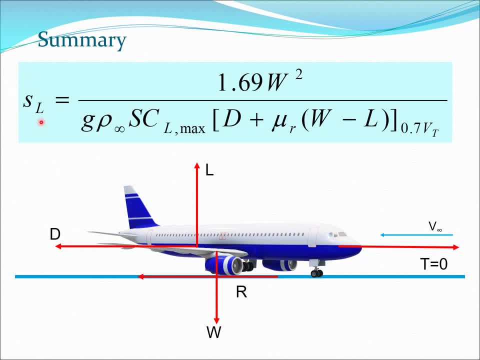 So let us summarize today's lecture. We derived this important equation sl and we clearly saw that this is directly proportional to w square. That means weight of the aircraft is very important at winds. we saw this is HUF, and we also saw that there are very many parameters such as density of air CL max D. 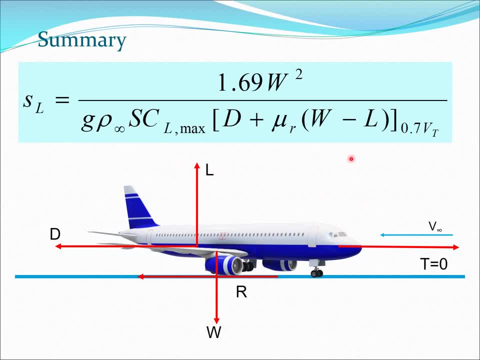 the l and mu r, which can be used to essentially control the landing distance for a given aircraft. So, depending on the altitude you are in, whether you are a hot day or not, you can potentially manage the situation. Also, remember that you can use spoilers to control. 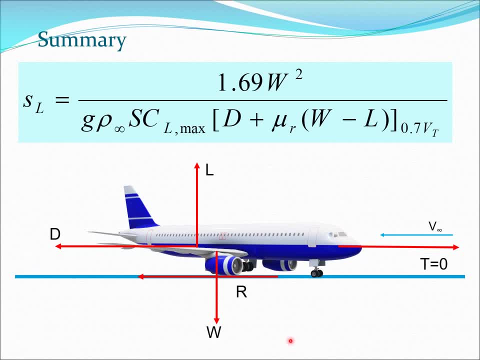 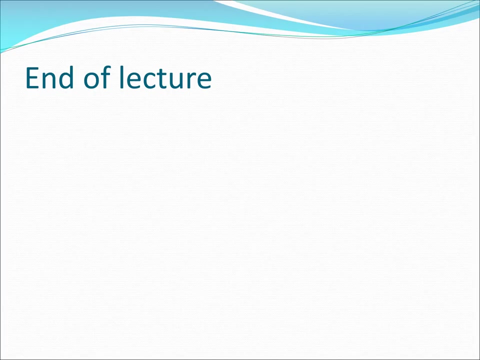 friction coefficient, mu r. So again, just recall, this was the basic diagram of the forces which act on the aircraft, and so, through the use of this diagram and the forces we were obtained to, we obtained this math model which gave us the landing distance. So I am going to end this lecture today. One important thing to leave you with is that 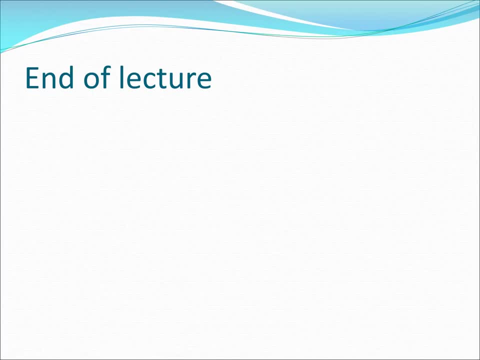 most of the accidents and problems which take place in aircraft take place during landing and takeoff, because these are the regions where the aircraft is very vulnerable. It is very near the ground, and so any mistakes by the pilot can result in catastrophic problems. So it is very important to be very careful when you are taking off, and even more careful 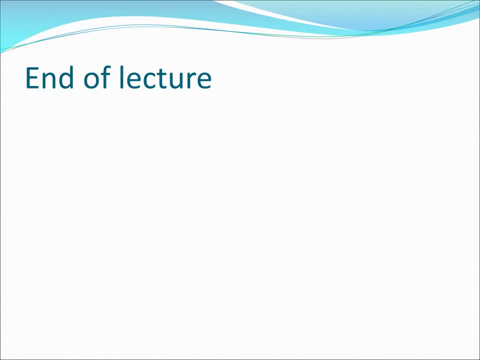 when you are landing, because these are the situations when you encounter low air velocity and you are actually touching back to the ground. So I will end this video here, and I think this is the end of this lecture. Thank you for watching. So this concludes a large part of the problem. where we discussed cruise, where we discussed 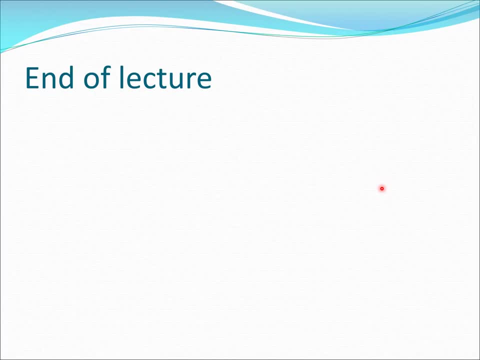 takeoff and landing, and next we are going to start looking at the V-N diagram or at turning flight. See you then.